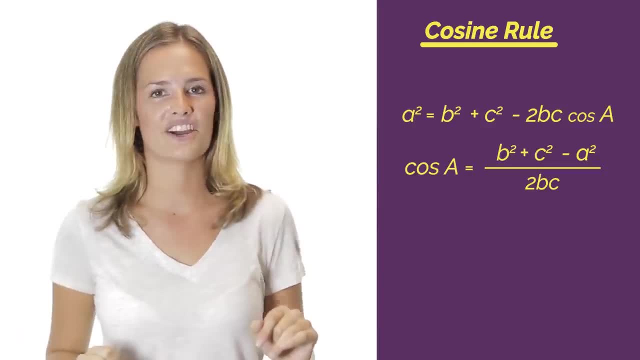 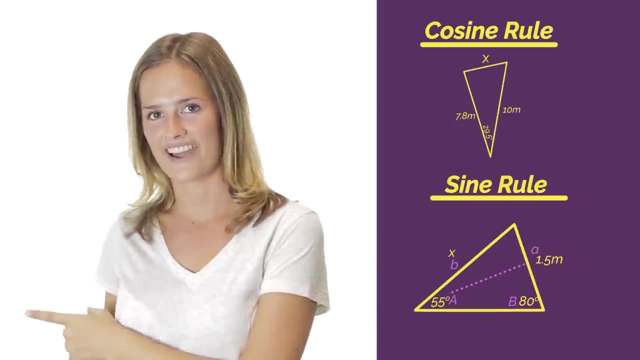 rule. We will look at how to use the cosine rule in the next video, but for now we are going to look at when to use the sine rule and when to use the cosine rule. Remember, in the sine rule video I said that you need to label the sides with little a. 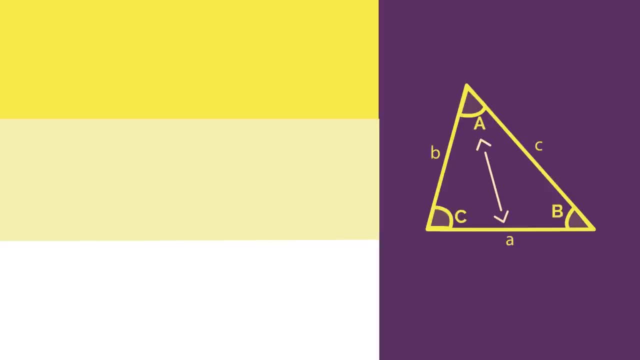 b and c's and angles with capital A, B and C's, and the side A and angle A are always opposite, side B and angle B are always opposite and side C and angle C are always opposite. This is really important. Both the sides are always opposite. 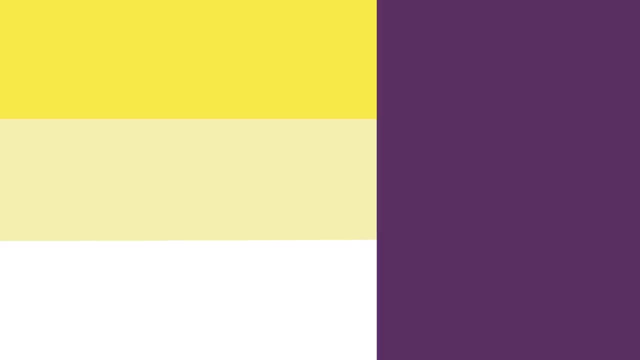 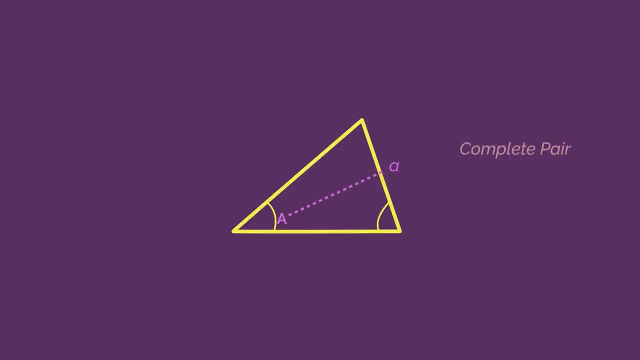 So when does the sine rule work? The sine rule works on pairs. You need one complete pair of a side and its angle and then you need half of the information of the other pair. So this is the complete pair and this is the half pair. We have the 80 degrees and we want 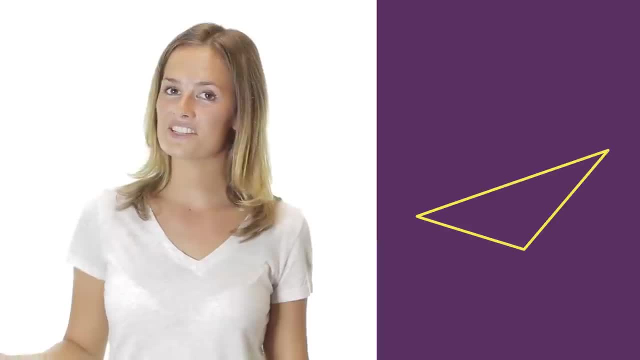 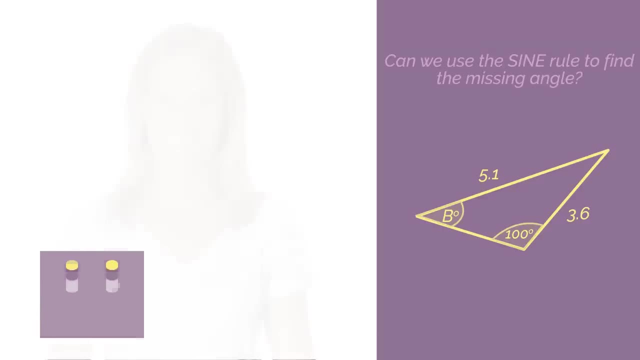 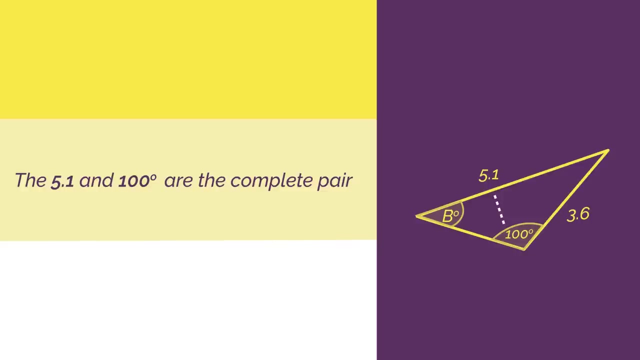 the side that is opposite. Can we use the sine rule to find this missing side? Yes, We can. The 5.1 and 100 degrees are the complete pair and the opposite, and the 3.6 and the missing angle B are the half pair. 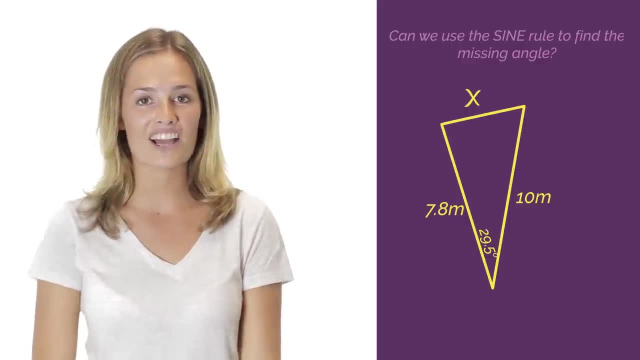 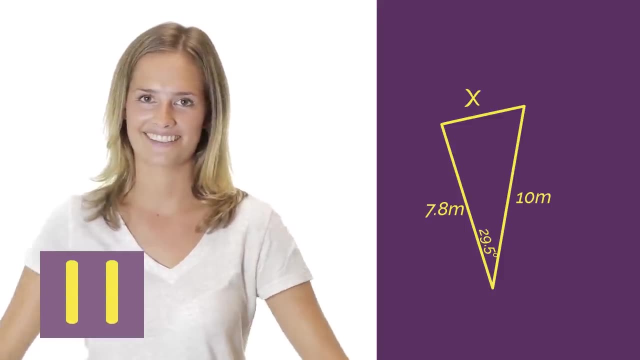 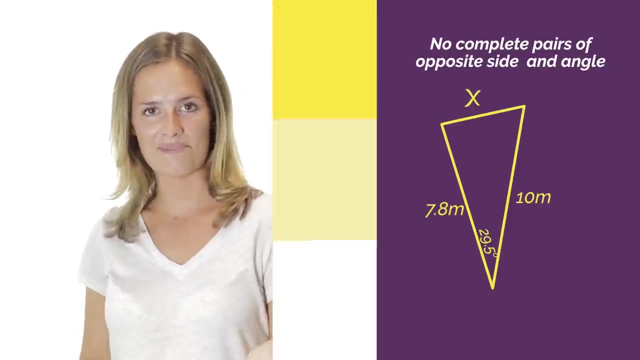 What about this triangle? Can we use the sine rule to find the missing side? Pause the video, work out the answer and click play when you are ready to check. We can. No, we can't. We don't have any complete pairs of opposite side and angle and the half pair. 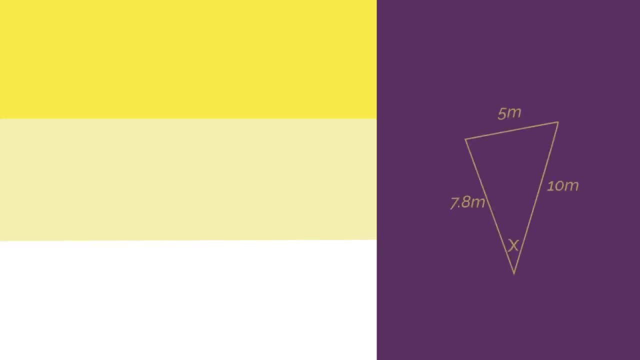 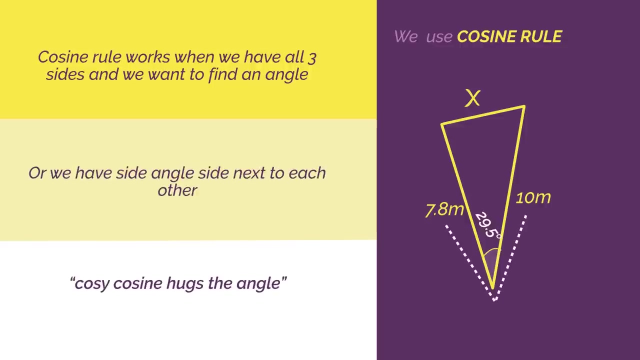 So this means we use the cosine rule. The cosine rule works when we either have all three sides and we want an angle, or we have side, angle side next to each other. Think of it as cosy cosine hugs the angle, Side, angle side. 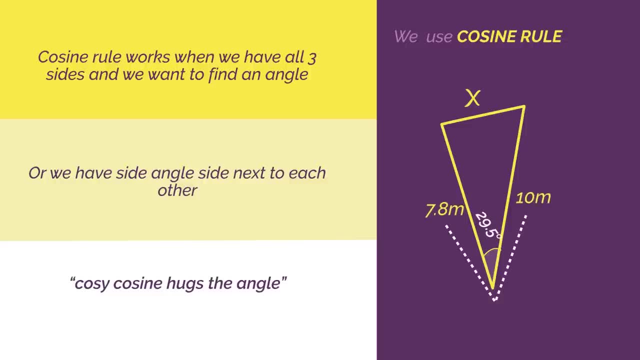 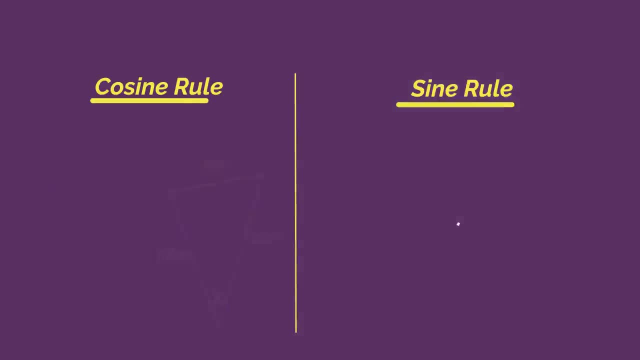 So from this video, you should know that if the triangle isn't a right angle triangle, we can use either the sine or the cosine rule to find the missing sides or angles. You should know that the sine rule needs one complete pair and half of the second pair, Whereas 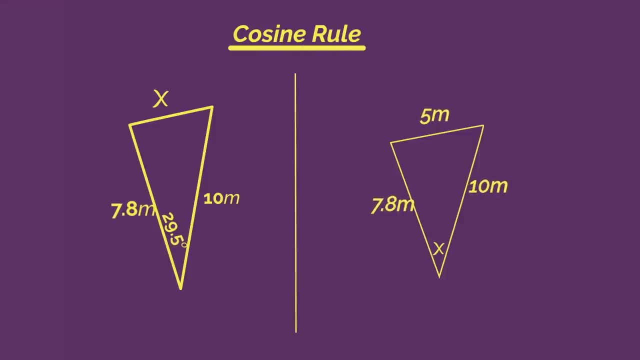 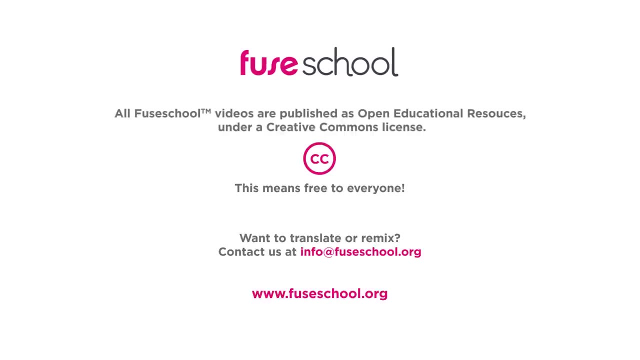 the cosine rule can either have all three sides given or side, angle side, So we've done that. Thanks for watching.